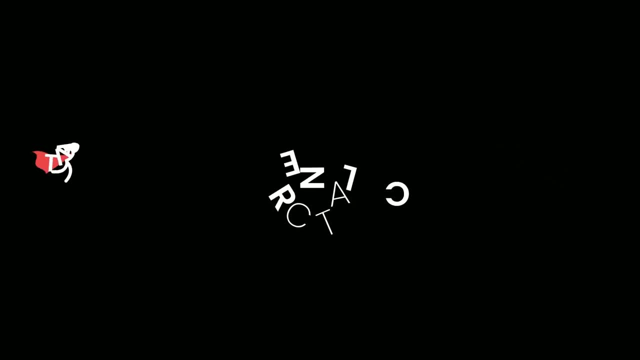 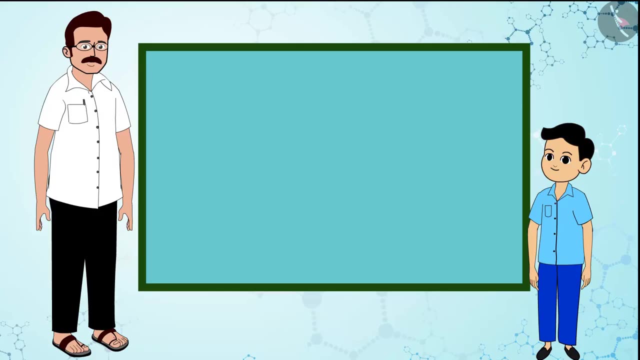 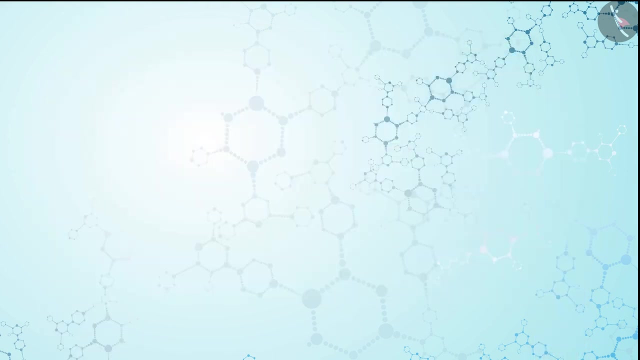 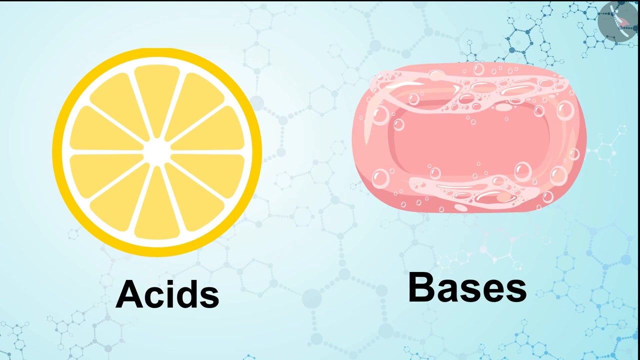 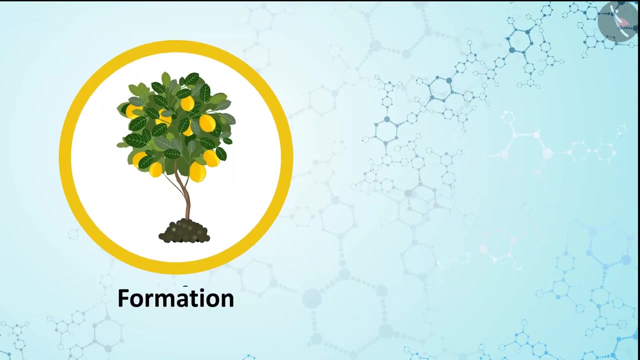 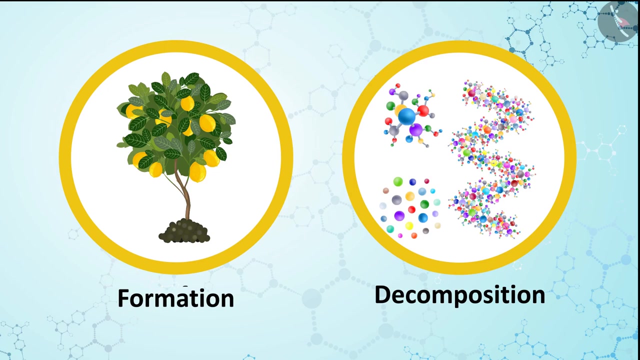 Hello children. acids and bases are encountered daily in our everyday lives. They are both an important part of our livelihood. They play an essential role inside or outside our body. From the formation of food to the decomposition of any substance, acids and bases have a role. 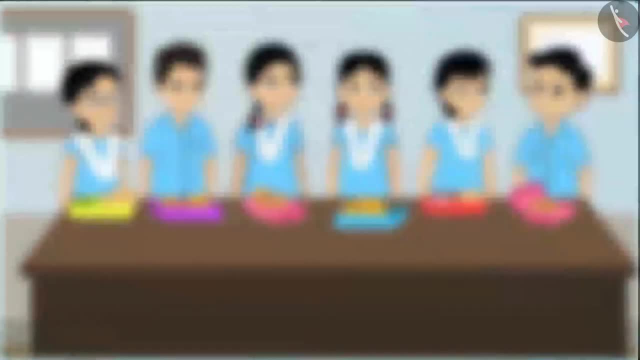 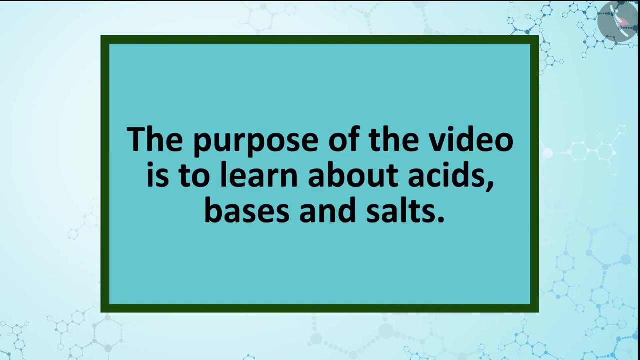 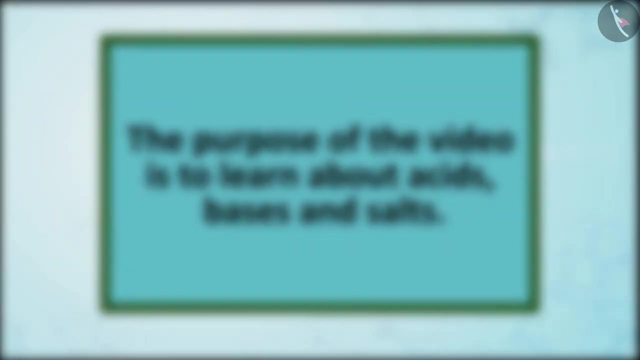 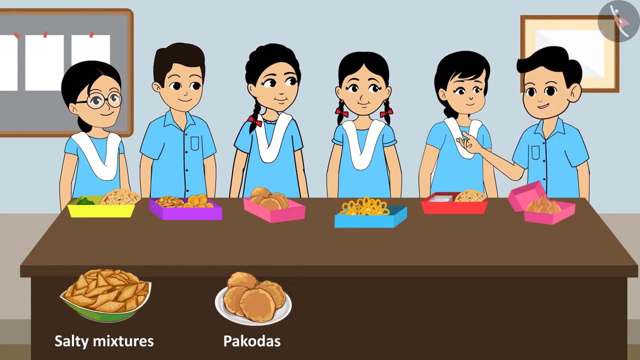 Let us know about their use in our daily lives. We will go to Raju and his friends to learn more about this. The purpose of this video is to learn about acids, bases and salts. Yesterday being a festival, my mother prepared salty mixtures, pakoras, samosa and a few sweets. 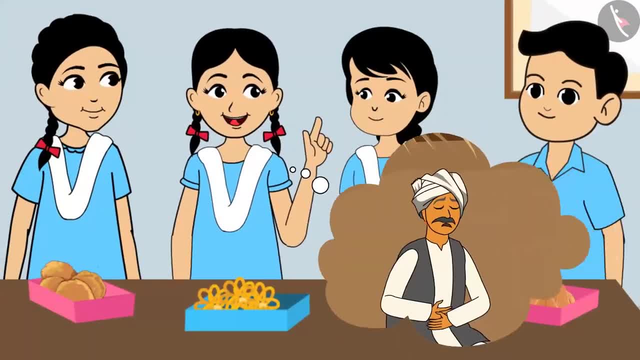 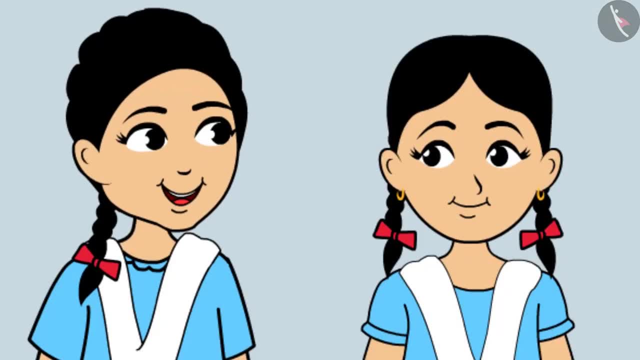 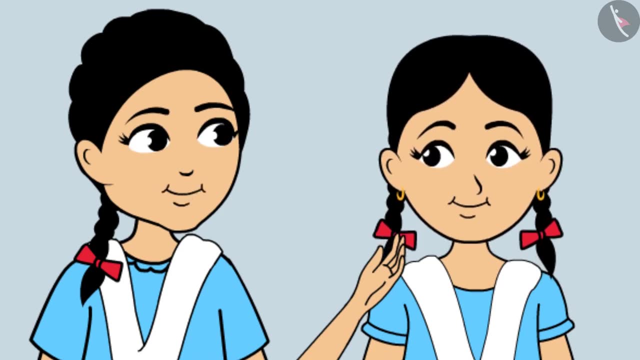 My mother has also prepared. However, my father fell sick in between with a lot of stomach ache and could not eat much. Wow Raju, what samosas your mother makes and her tamarind chutney. it is so tangy, spicy. 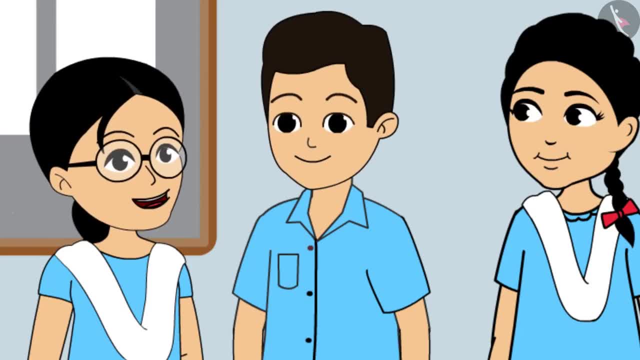 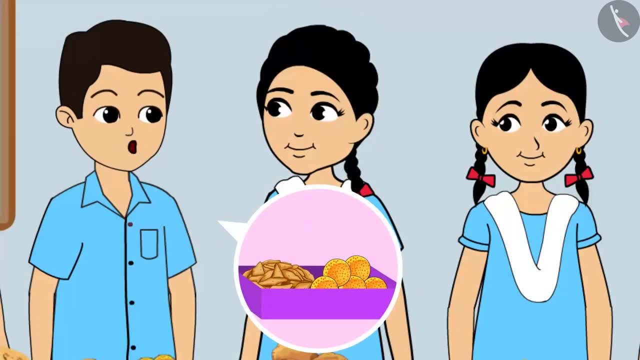 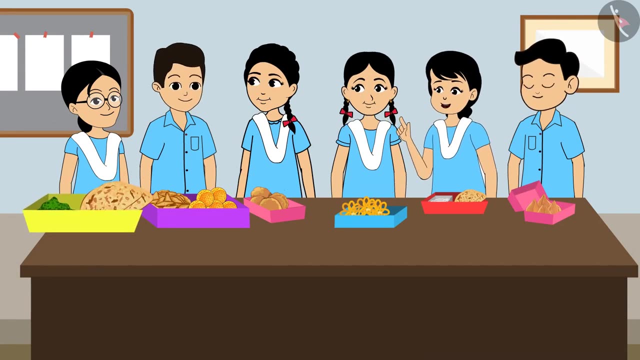 and tasty. My food is slightly bitter. My mother gave me the green leafy vegetable curry with the roti. I brought laddus and a little mixture. Wow, a few brought sweets, a few rotis, few green leafy vegetable curry, and I brought 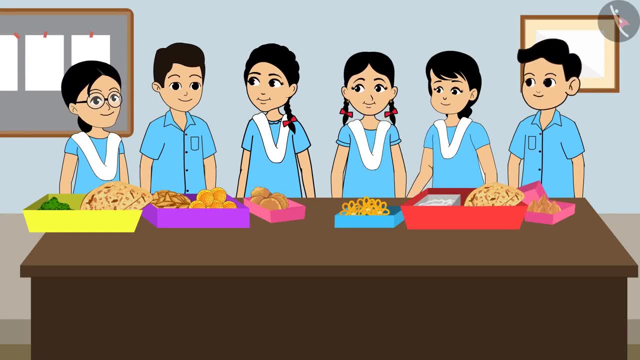 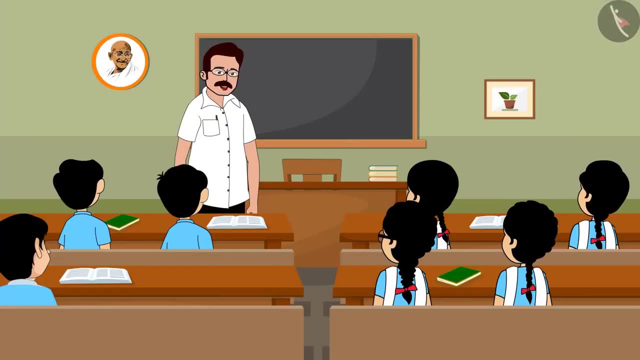 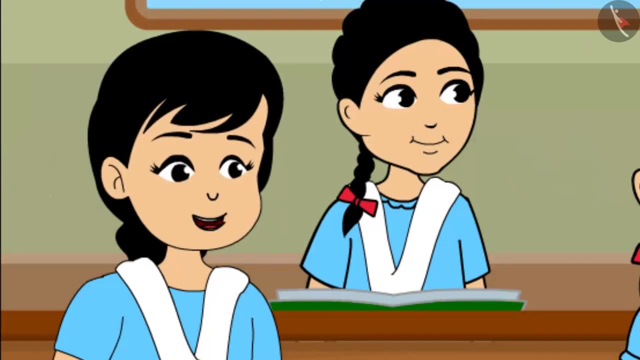 parathas and curd. Let us eat quick and share the delicious food. We have science class immediately after the lunch break. Good afternoon, children. did you all have your lunch? Yes, sir, Today we brought food with different tastes: some sour, some sweet, some salty and some. 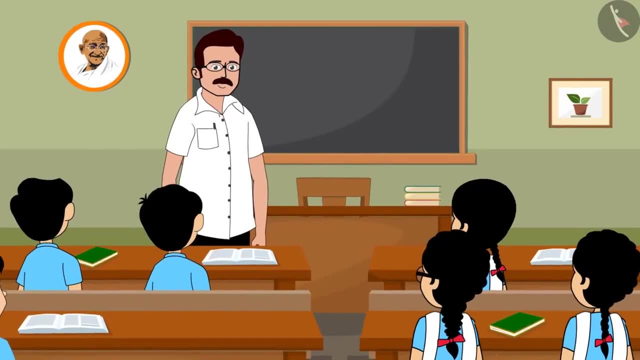 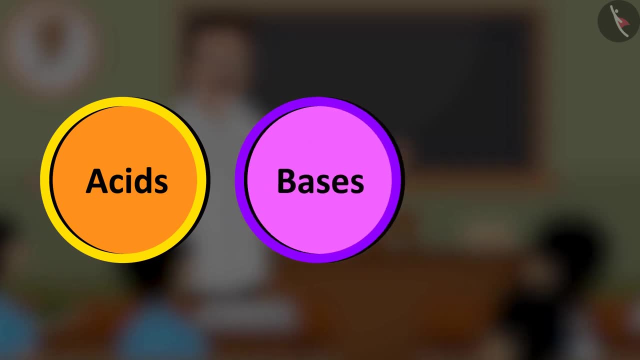 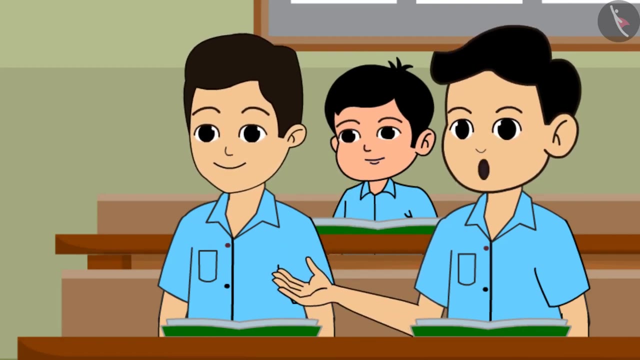 bitter Children. do you all know that different foods have different tastes because of a lot of food contains acids, bases and salts, Acidic. I heard that acids are different. Yes, sir, Not all acids are dangerous, Lata was telling me yesterday. Oh no, not all acids are dangerous. Mamta, make a list of the foods you eat that are mostly sour: Tamarind chutney, orange tamarind, curd, samosa, guava apple and That's enough. 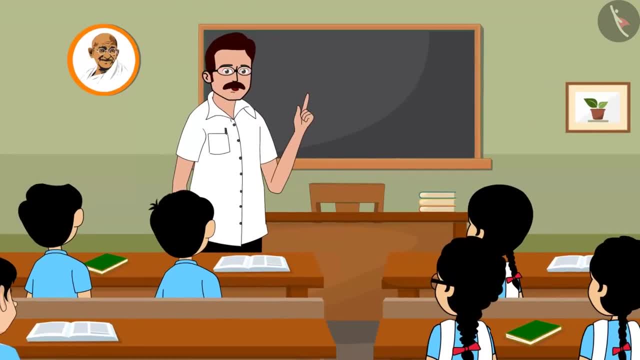 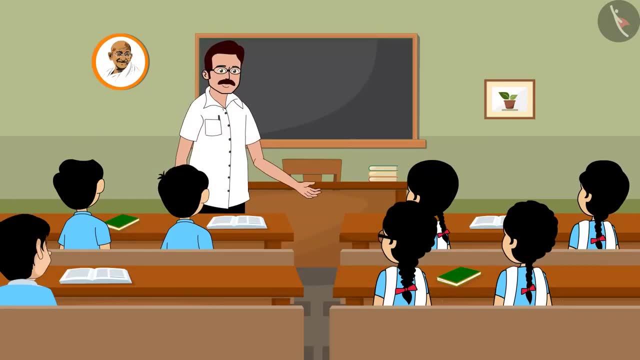 Thank you. Do you know? Do you know? Do you know? We contain acids which cause sourness in them, Acid in our foods? Yes, all these are natural acids. What happens when you eat food? It gets digested. 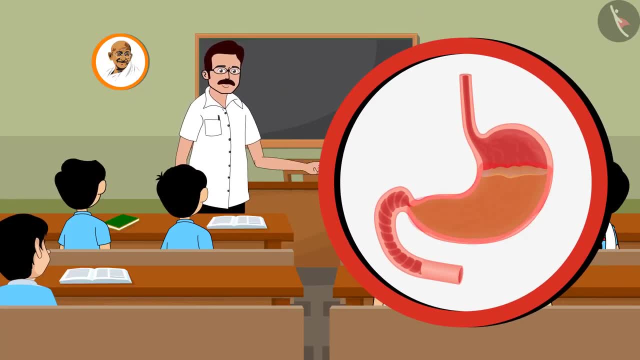 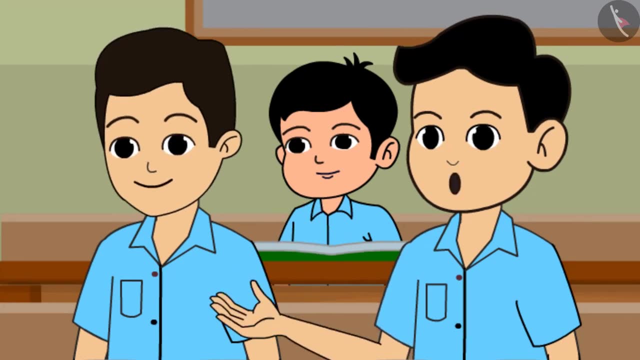 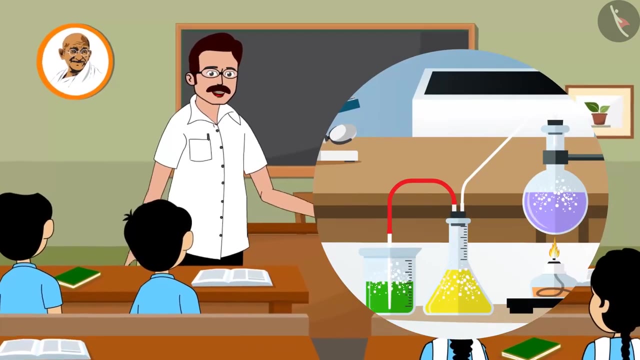 Yes, Your body also produces some acids and they help in digestion of food, I see, so there are some good natural acids as well. Yes, The acids that are there in our school's lab are very powerful and dangerous and need to be used with caution. 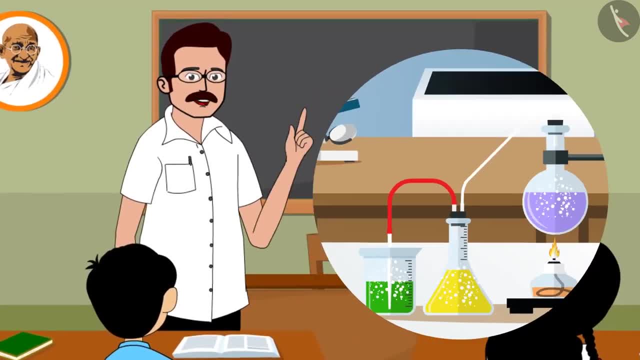 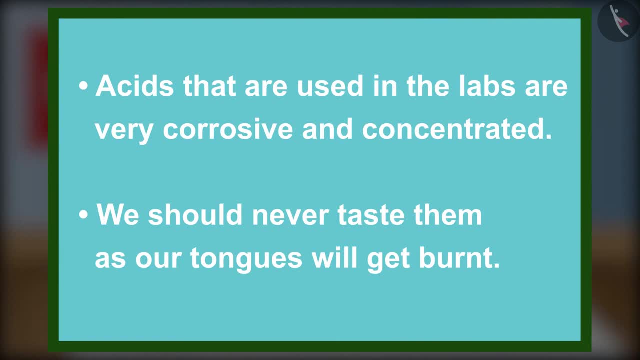 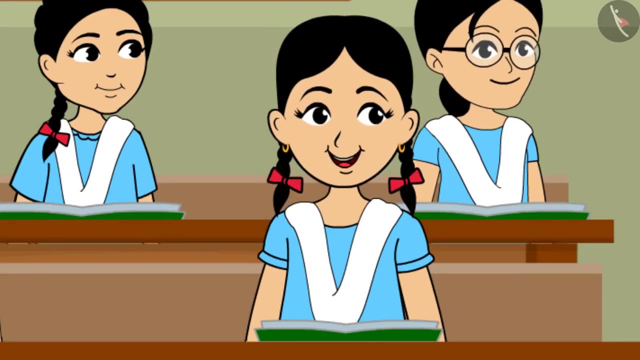 They are high in acidic content and low in water content. Children, the acids that are used in the labs are very corrosive and concentrated. We should never taste them, as our tongues will get burned. Sir, my father had stomach pain yesterday. When we went to the doctor he said my father had acidity. He gave him some medicine. He said it was some antacid. Sir, does the medicine nullify the acids? Yes, Due to spicy food and also flatulent food, stomach becomes acidic And due to this people have acidity. If we take antacids, at that time we get relief. 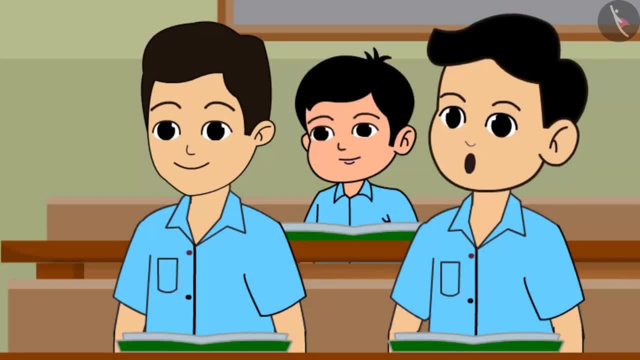 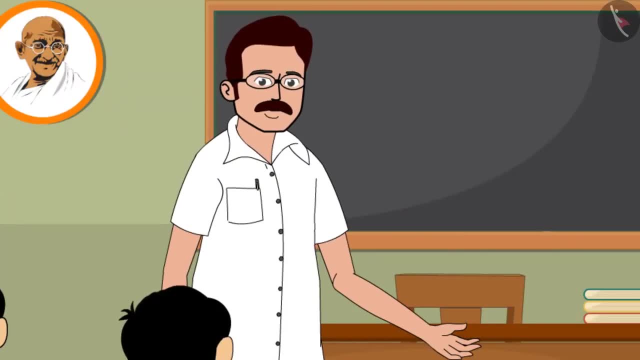 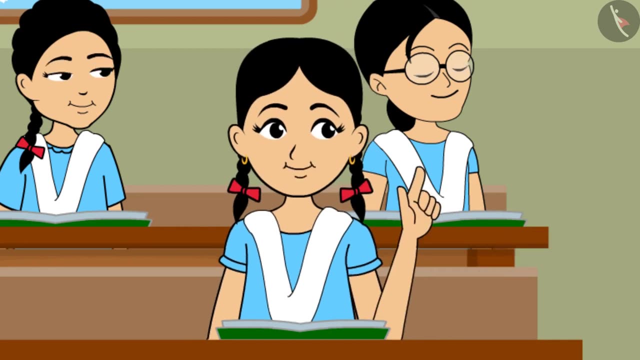 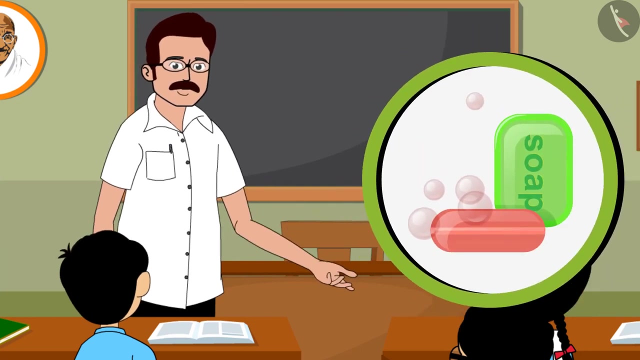 Antacids have bases. Do bases nullify the effect of acids? Yes, We shall talk about this tomorrow. My father was feeling better after two hours yesterday after he took the medicine. Bases are the chemical compounds which are soapy in touch and are not usually meant for human consumption. 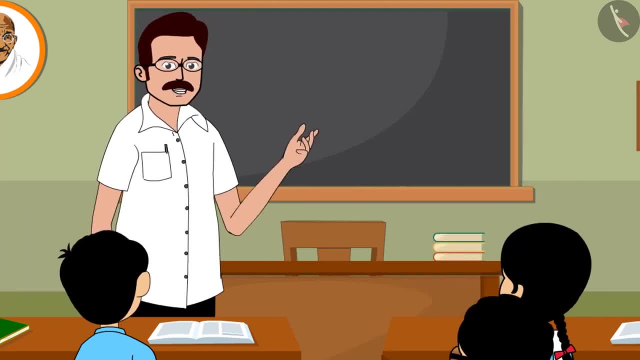 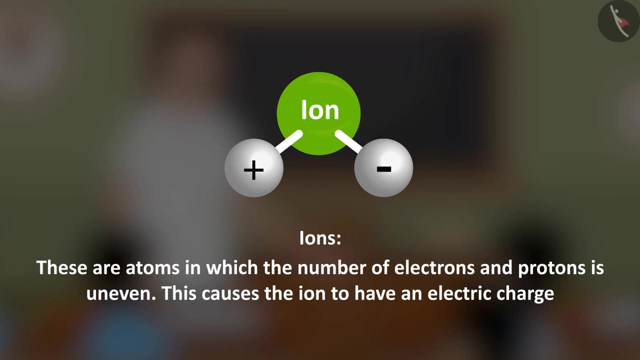 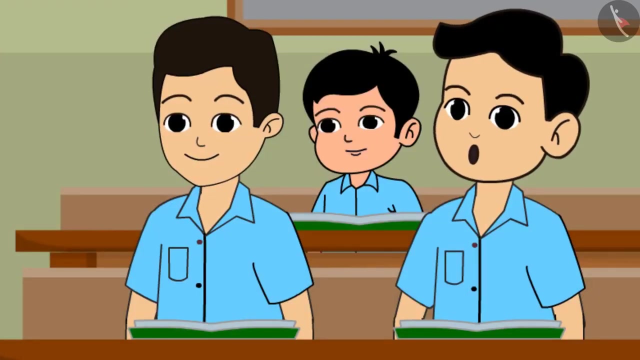 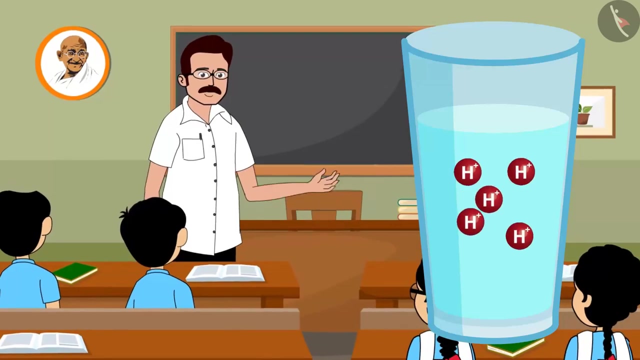 They are bitter in taste. They have a wide range of applications in our daily life. They have hydroxide ions present in them and acids have hydrogen ions present in them. Sir, can you please explain in detail? When acid dissolves in water, it releases hydrogen ions. 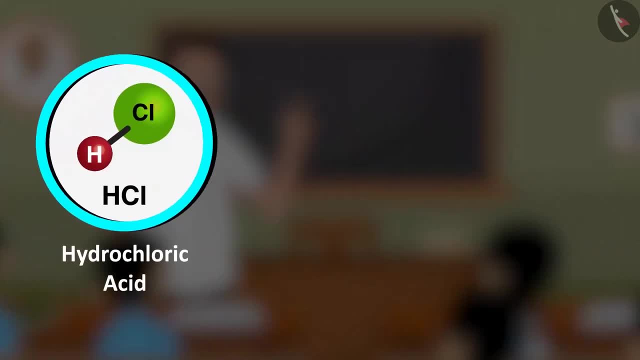 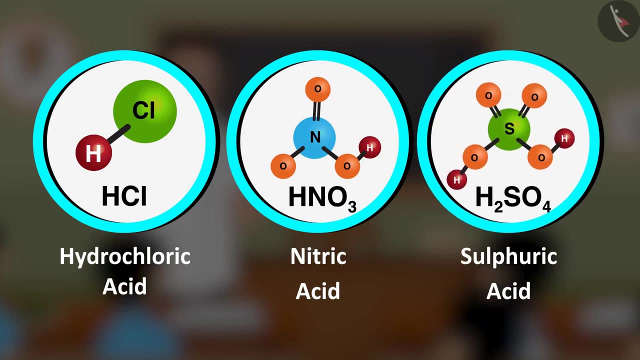 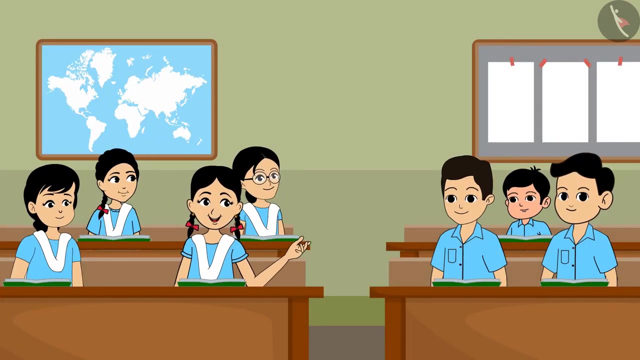 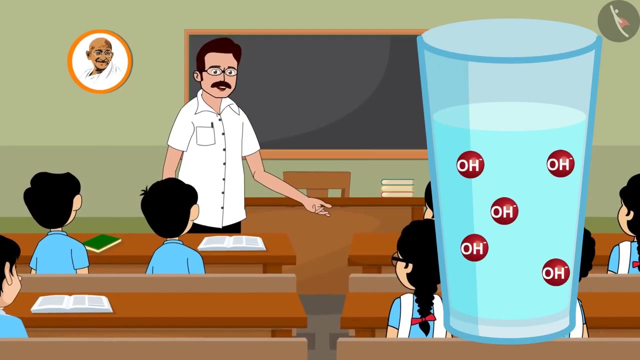 Acids have hydrogen in them, Like HCl, Hydrochloric Acid, HNO3, Nitric Acid, H2SO4, Sulfuric Acid, etc. Sir, do bases have more hydroxide ions in them? Base is any compound that yields hydroxide ions when dissolved in water.